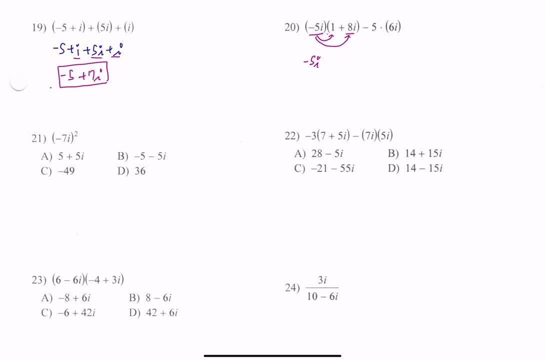 Negative 5i plus 8i, which is negative 40i squared, And then you distribute negative 5.. Actually, you multiply negative 5 and 6i, which is negative 30i. All right, Whenever you simplify powers of i, you should use i squared right. 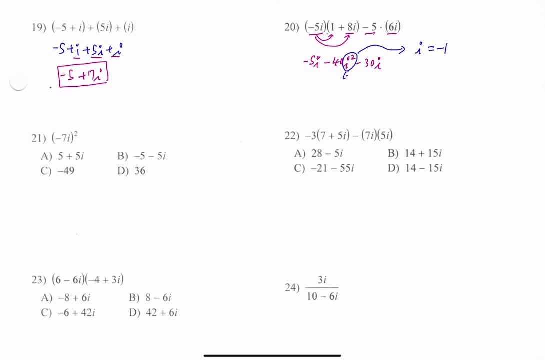 i squared is equal to negative 1.. So Plug in negative 1, for i squared Negative 1 times negative 40.. Positive 40. And then you add these two numbers, Negative 5i plus negative 30i, which is negative 35i. 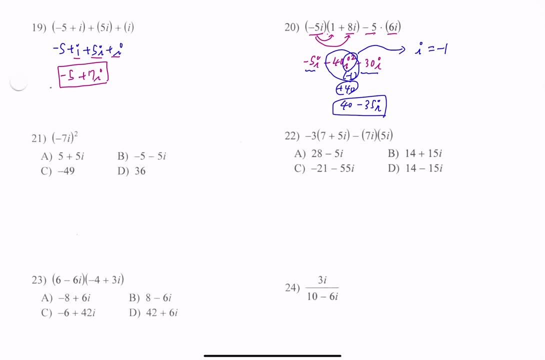 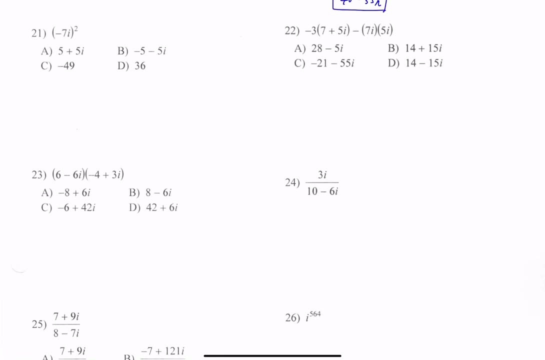 And then you keep 40 in the front. Next, Parenthesis: negative 7i squared, Which means negative 7.. Squared times: i squared. Parenthesis: negative: 7 squared is 49.. i squared is negative 1.. So negative 1 times 49, negative 49.. 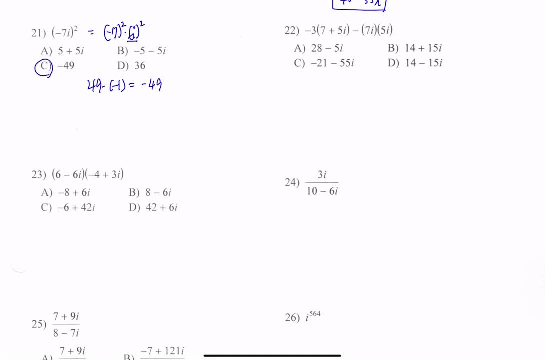 C 22.. You distribute negative 3 for these two numbers first, And then you multiply these two: Negative 3 times 7, negative 21.. Negative 3 times 5i. Negative 15i. Negative 15i. 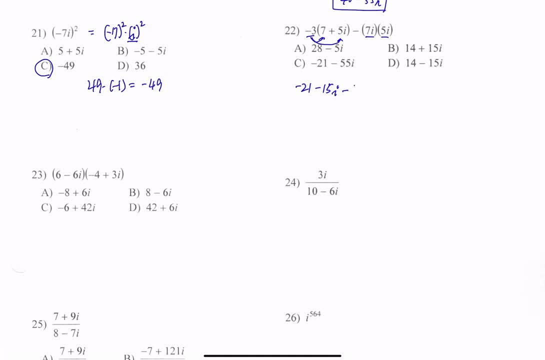 And then minus 7i times 5i, 35i squared. i squared is equal to negative 1.. So negative 1 times negative 35, positive 35.. 35 plus negative 21 is 14.. Yeah, 14.. 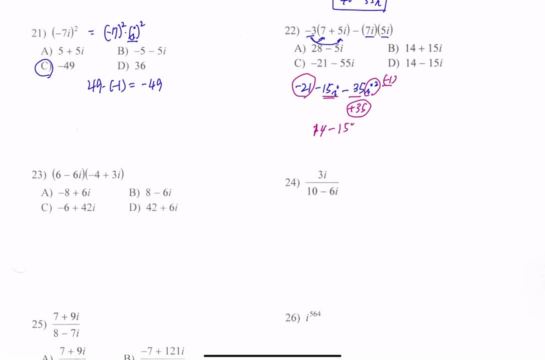 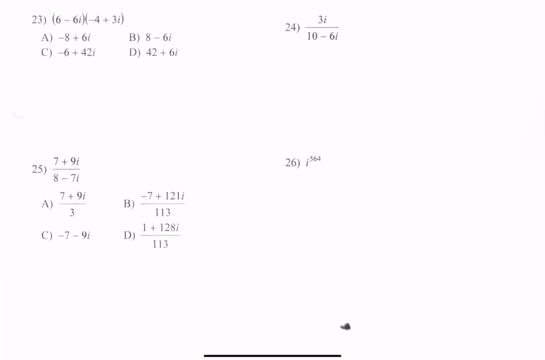 14 minus 15i, Number 23.. Binomial times binomial, So you should use FOIL way: FOIL: 6 times negative 4, which is negative 24.. 6 times 3i, 18i. 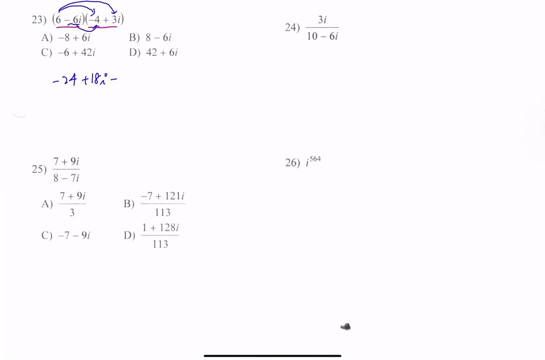 Negative 6i times negative. 4, positive: 24i. Negative 6i times 3i negative. Negative 6i times 3i negative: 18i squared I squared is equal to negative 1.. Negative 1 times negative: 18 is positive 18?. 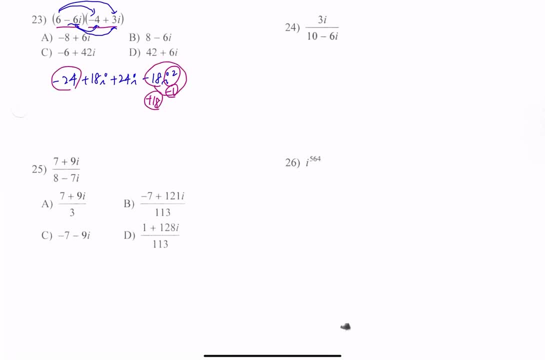 18 plus negative 24 is negative 6.. and then you add these two like terms because they are imaginary numbers. So 42i is 4ed to i, So negative 6 because negative 24.. Negative 6 plus 42i is the answer. 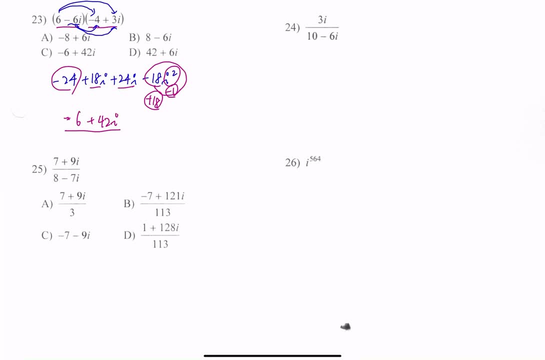 Number 24.. Okay, If there is binomial in denominator, to simplify this fraction, you should multiply complex conjugate of denominator, which is 10 plus 6i. You multiply 10 plus 6i in numerator and denominator In denominator to simplify this form. 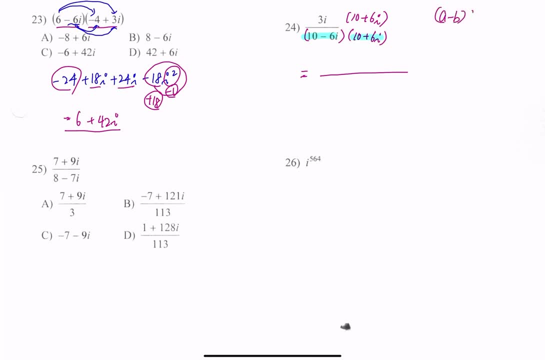 we need to use this a minus b times a plus b form, which is a squared minus b squared. So denominator will be 10 squared minus 6i squared. In numerator you just distribute 3i for these two terms. 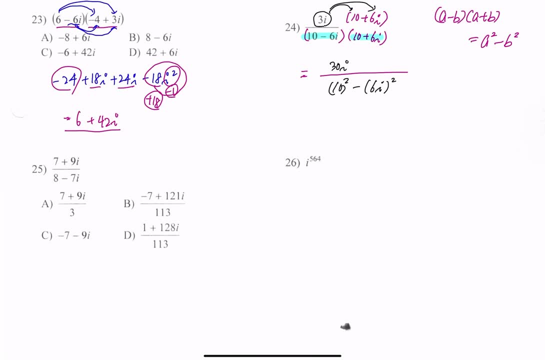 So 3i 3i times 10, 30i, 3i times 6i, 18i squared. Simplify more. Numerator i squared is negative 1.. Negative 1 times 18 is negative 18.. 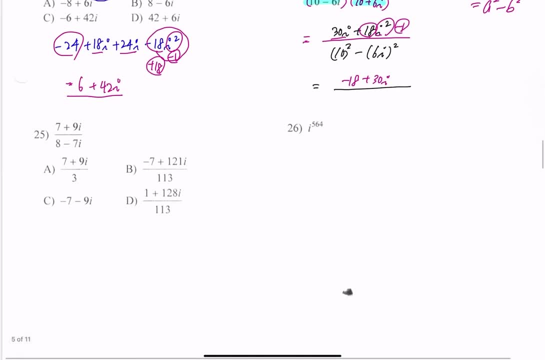 You keep 30i In denominator 10, squared is 100 minus 6, squared is 36.. i squared is: i squared which is negative 1.. So denominator, Denominator is 100 minus 36, negative 1, plus 36.. 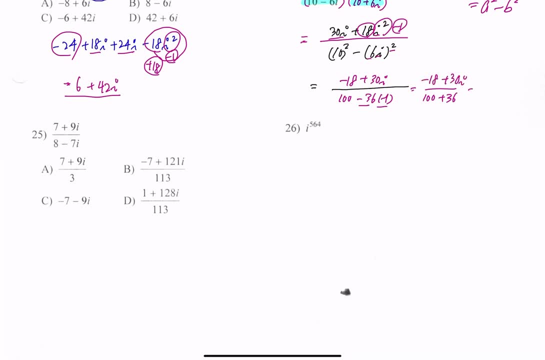 Negative 18 plus 30i. So denominator is 136.. Numerator negative: 18 plus 30i. This is yeah, all numbers are. all of these numbers are even numbers, So you can divide all of those three numbers. 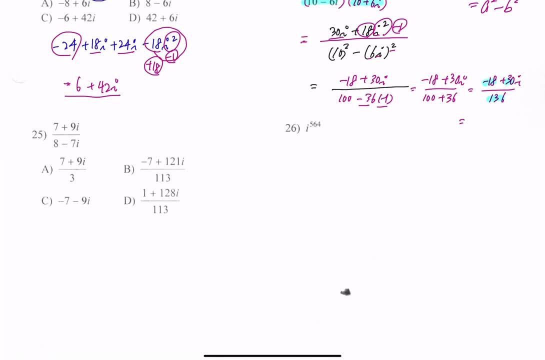 So you can divide all of those three numbers By 2.. All right, So 136 divided by 2, 68.. 18, negative. 18 divided by 2, negative, 9.. 30i divided by 2, 15i. All right. 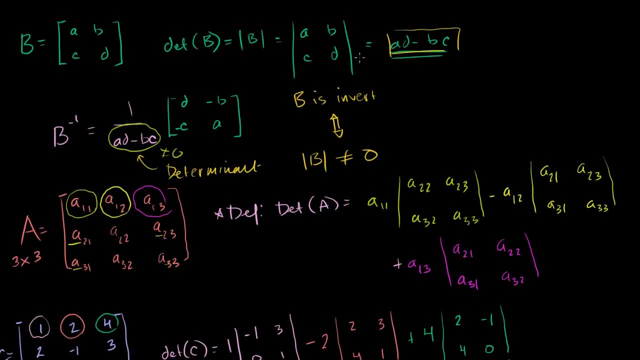 So far, we've been able to define the determinant for a 2 by 2 matrix. 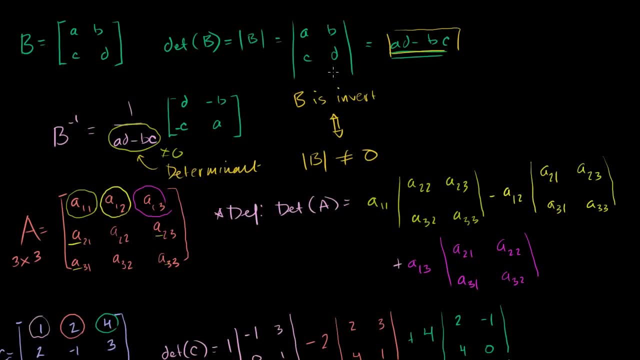 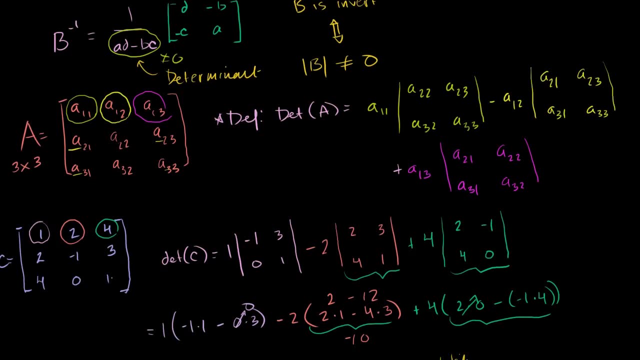 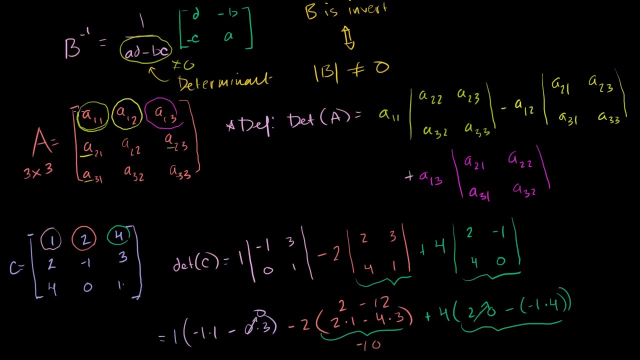 This is our definition right here, ad minus bc. And then we were able to broaden that a bit by creating a definition for the determinant of a 3 by 3 matrix, and we did that right here. We did that right here, where we essentially said the determinant is equal to each of these terms, you could call these maybe the coefficient terms, times the determinant of the matrix. 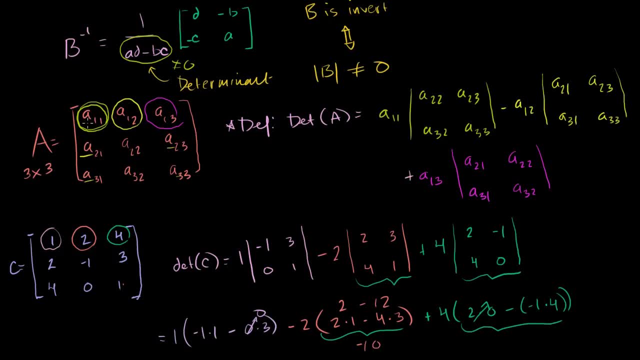 You can kind of view it as the sub-matrix produced. When you get rid of each of these guys, column and row. So when you got rid of this guy's column and row, you're left with this matrix. So we said this guy times the determinant of this. And then we kept switching signs, minus this guy times the determinant if you remove his column and his row. So it was left with these terms right there to get that determinant. 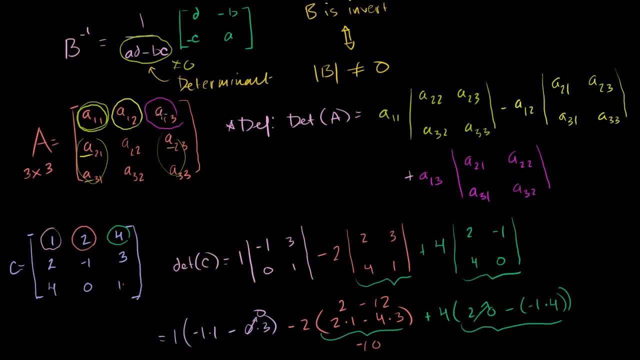 Then finally, you switch signs again, so plus this guy times the determinant of the 2 by 2 matrix if you get rid of this row and this column. 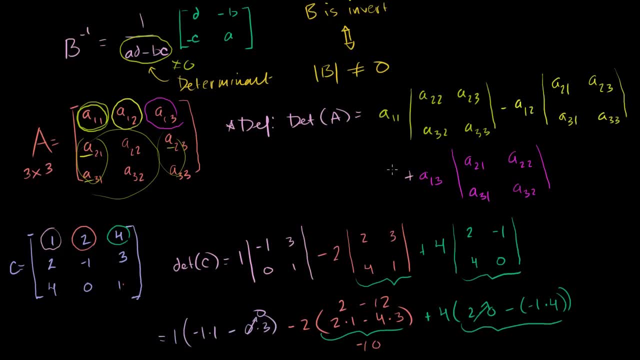 So it's this thing right here, which was this matrix. Now let's see if we can extend this to a general n by n matrix.